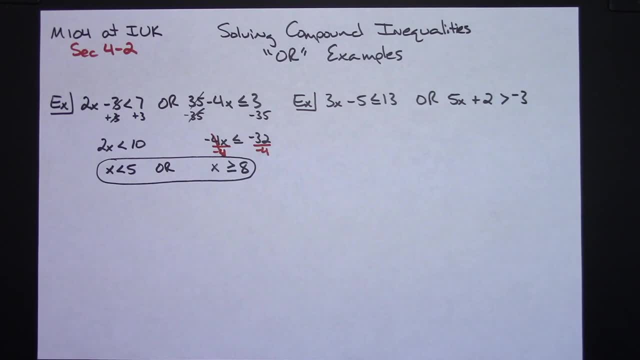 down and put this solution in interval notation. Alright, now, probably the easiest way to do this on ORs is to picture it on a number line and just see what happens. Okay, so let's draw a number line, Let's put 5 and 8 on the number line, because those are the 2 that we've 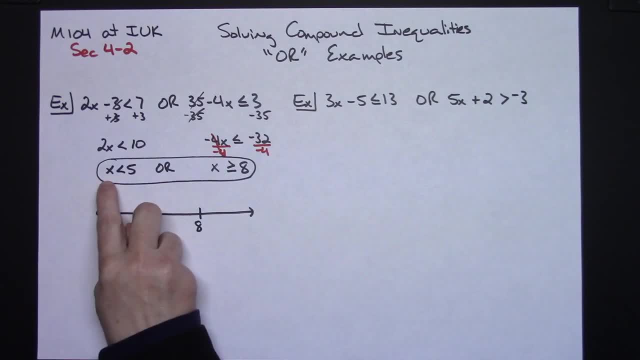 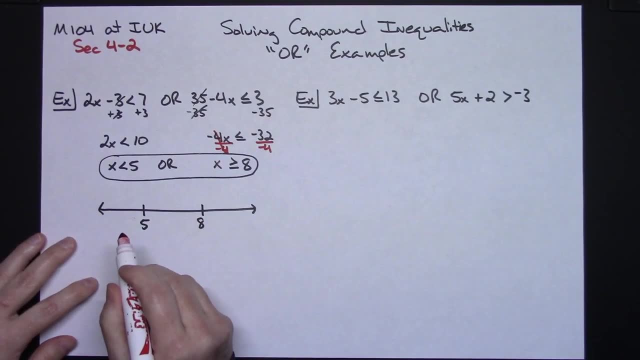 got here, all right, and then let's just graph it and see what it looks like. this says x is less than 5. all right, well, that would be down here, okay, and less than 5 means I'm not going to include 5 in my answer, so curvy bracket there, and that part of the equation is here. all right now. this says x is: 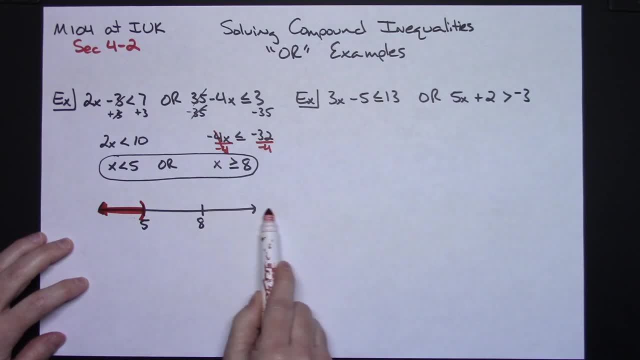 greater than or equal to 8. well, those would be these numbers over here. the equal to part says that I'm going to include 8 in my answer, so I'm going to have a square bracket there and shaded this way. all right, so on a number line pictured, that's what my ors look like. okay, now, if you are. 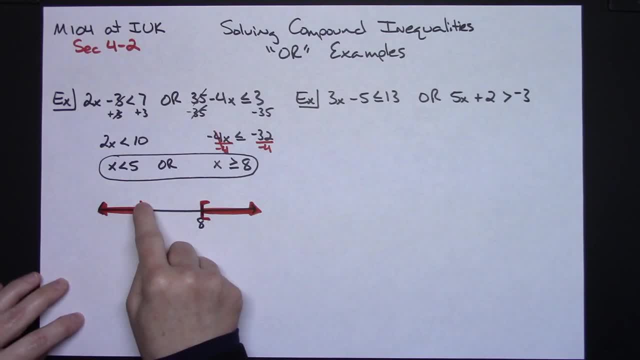 in a high school class, or say an algebra 2 class in high school, algebra 1, you could- would not necessarily be using the interval notation with the square bracket and curvy bracket. you might be using open and closed dots, where this would be an open dot and this would be a. 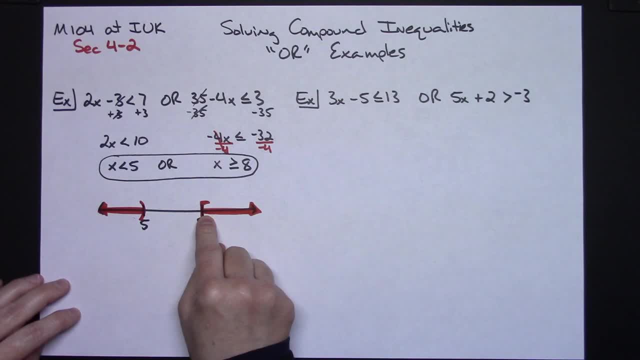 closed dot. The concept's the same: Square bracket or closed dot means that we are going to include the number in the solution. A curvy bracket or an open dot means that we would not be including the number in the solution. Okay, so a solution here in terms of interval notation. Okay, we all. 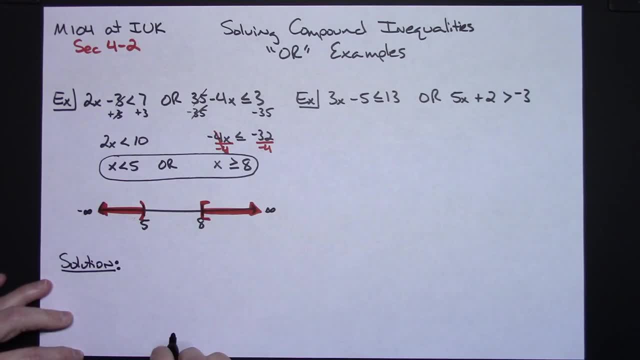 know that negative infinity is down here on the number line. Positive infinity is here on the number line. Okay, so curvy bracket. negative infinity all the way up to 5.. Curvy bracket on 5. because I do not want to include it, I'm going to skip over this section of the number line. 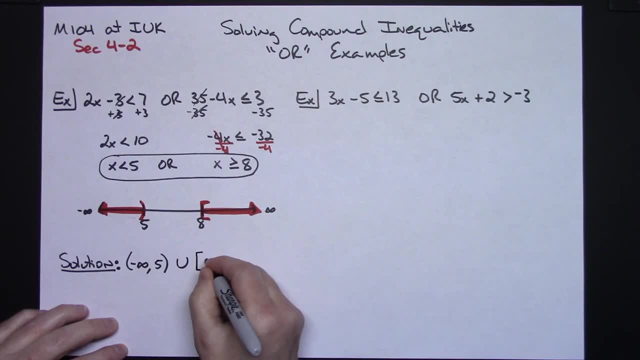 so I'm going to union. I want to include 8,, so square bracket and then all the numbers up to positive infinity. Okay, if you are not, let's go ahead and write interval notation. If you are not familiar with interval notation, I'm sure there's some videos on my channel where I 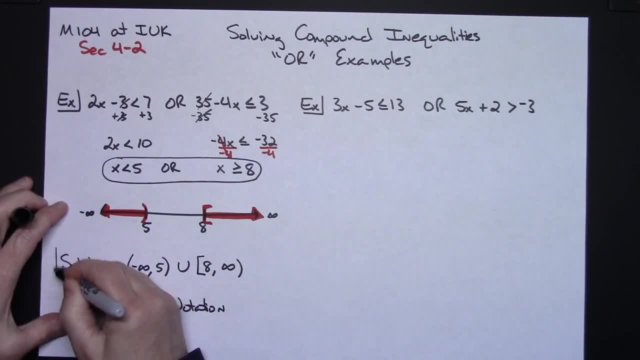 go into detail about explaining interval notation, okay, but in a college algebra class you're probably going to have to be writing that solution using your interval notation. all right, now let's just go ahead and do a second example here, because, while they look like they're going to be relatively 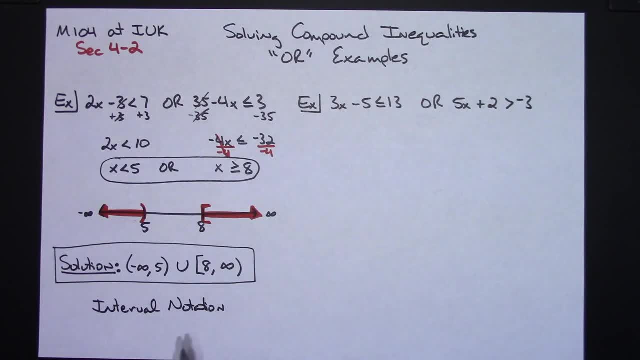 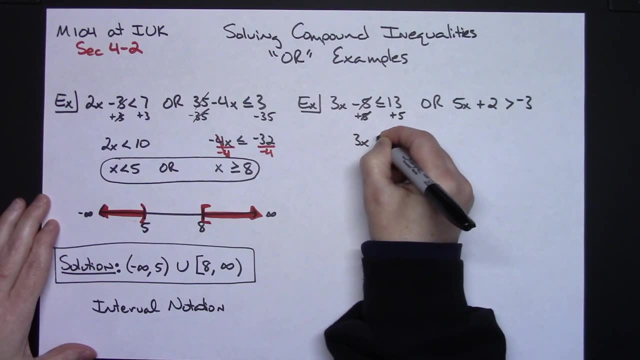 similar. you don't know necessarily what you're going to encounter until after you solve it. all right. so let's add five here to both sides of the equation to start solving this. i'm going to have a 3x is less than or equal to an 18. going ahead and dividing by that 3, i'll have x is less. 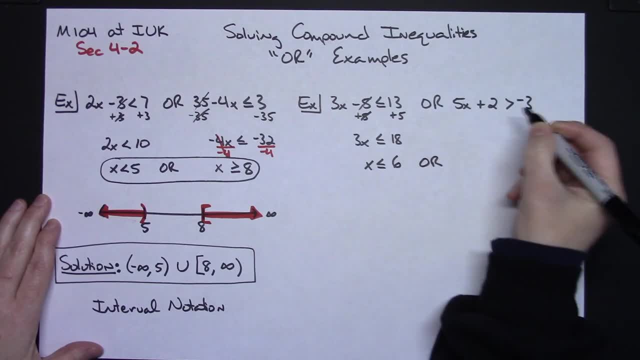 than or equal to 6. i'm going to go ahead and put my or in now solving this inequality. we'll subtract 2 from both sides of the equation. i'm going to have a 5x is greater than a negative 5. all right, dividing by 5 there does not mean anything, so i don't have to flip the sign or anything. x is: 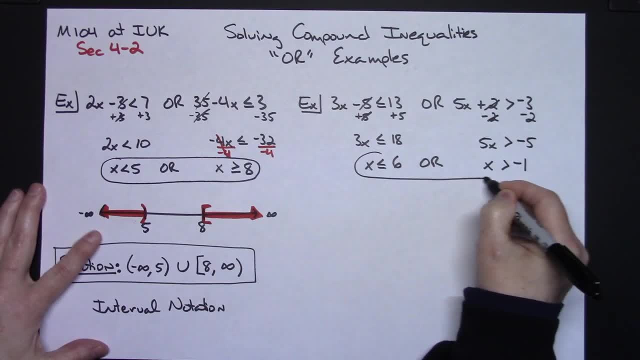 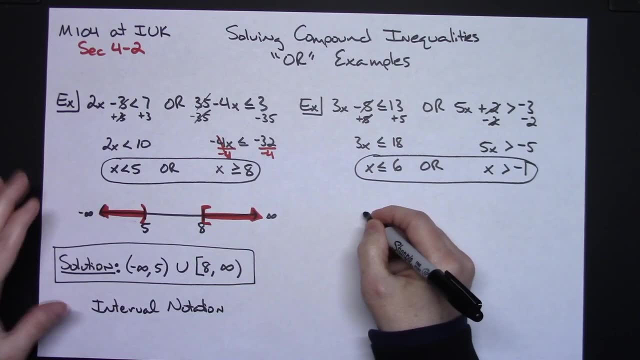 greater than negative 1. okay, so again, depending on what class you're in and what the expectations are, you might have to do that. so i'm going to go ahead and do that, and i'm going to go ahead and might possibly be allowed to leave your answer like that. all right, but let's go ahead and write. 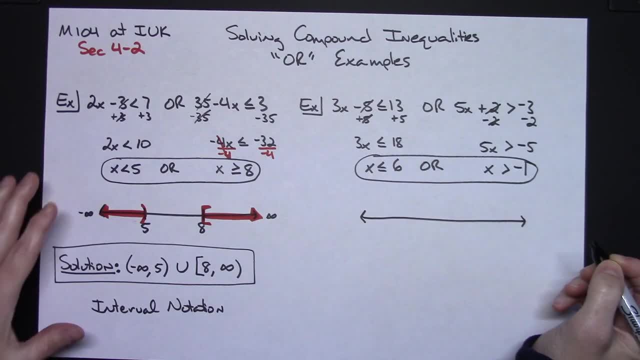 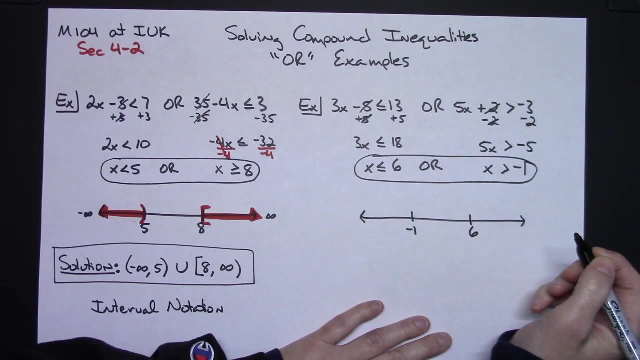 it in interval notation. let's draw it on the number line first and see what it looks like. i have a negative 1 to 6, clearly negative. 1 has to be down here. 6 has to be down here somewhere, all right. so this says x is less than or equal to 6. all right, so here's 6, the numbers that are less. 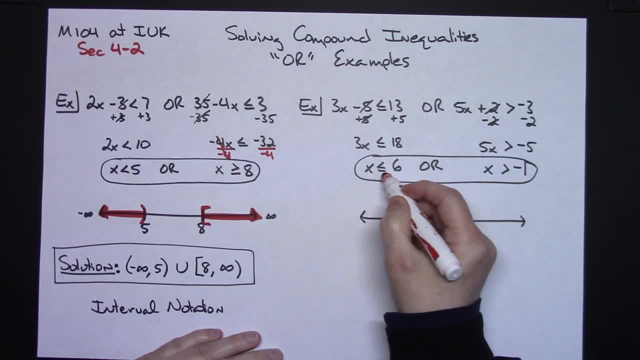 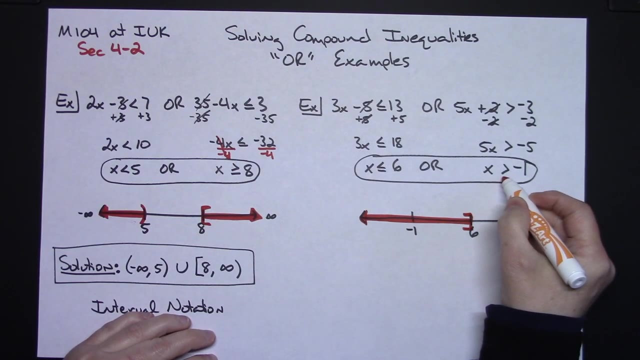 than 6 are this way, so let's shade that less than or equal to means i do want to include 6 in the answer, so square bracket and it's going to be all of these numbers right here. okay, now let's go ahead and do this one. it says x is greater than negative 1. okay, so x is greater than so. i'm not including 1. 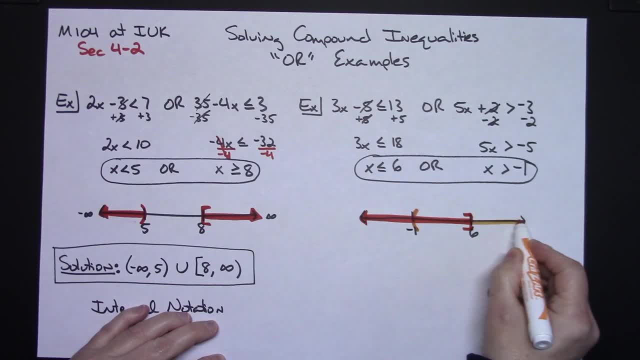 but the numbers that are greater than negative 1 would be all of these numbers and, as you can see, the whole entire number line got shaded. now, granted, yes, this is an open dot on negative 1. so if i'm going to do this, i'm going to do this, and i'm going to do this, and i'm going to do this.